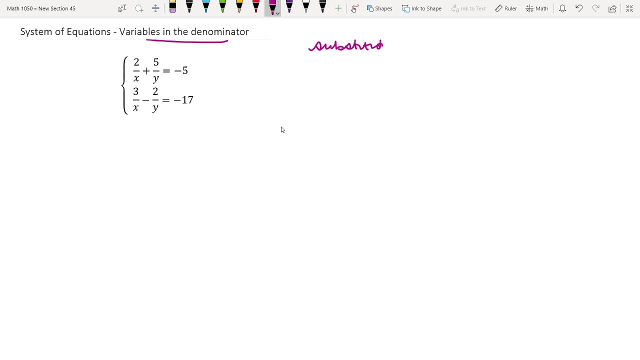 going to use a substitution method, Okay. so I am going to say: well, notice that in both situations the X is on the bottom and the Y is on the bottom. So I'm going to say, what if in just a random variable, let's say that A here actually represents the idea? 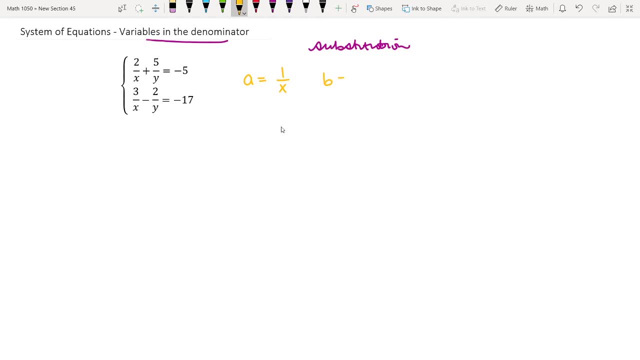 of having X in the denominator, And then I'm going to say: B is when Y is in the denominator. What it's going to allow me to do is to rewrite the equation without this. So, in place of the X in the denominator, I'm going to pull here, I'm going to pull here and I'm going. 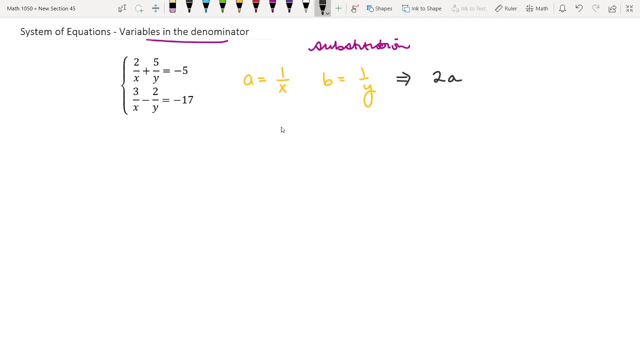 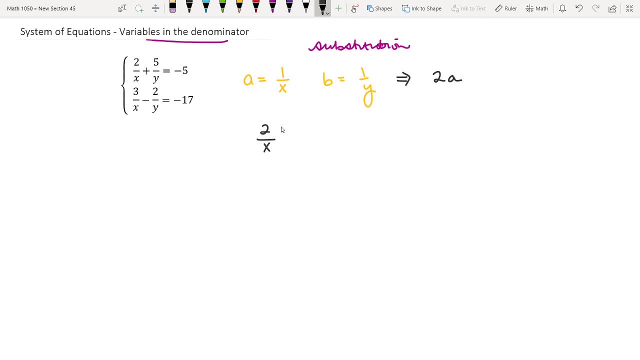 is. I'm saying here's this, and I'm going to, if you would, I'm going to divide out the one over X. Well, we know, with fractions what I'm doing: there is timesing by the reciprocal and that cuts out that value, Okay, So of course, this here was a maybe. 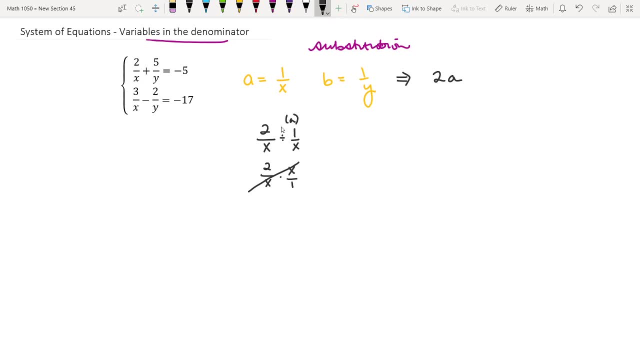 and so when we're doing all that kind of thing, we're essentially saying: I'm getting rid of you and I'm putting you in place of it. Now, that makes it a little bit easier to look at this next one, because I'm saying in place of the y in the denominator I'm just going to put. 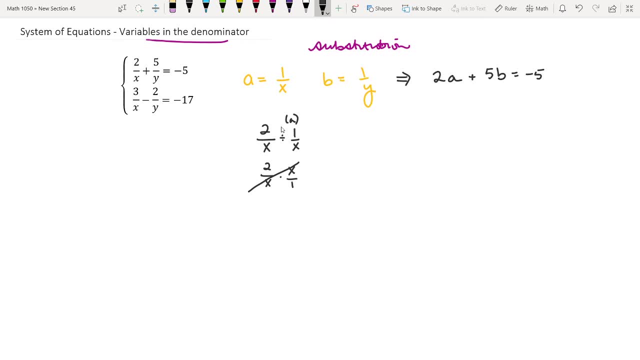 a, b, And then I can do the same thing here with the bottom one and say 3a minus 2b equals a negative 17.. And now I have a more typical arrangement that we use to a system of equations and we can go ahead and solve for that, If you recall. 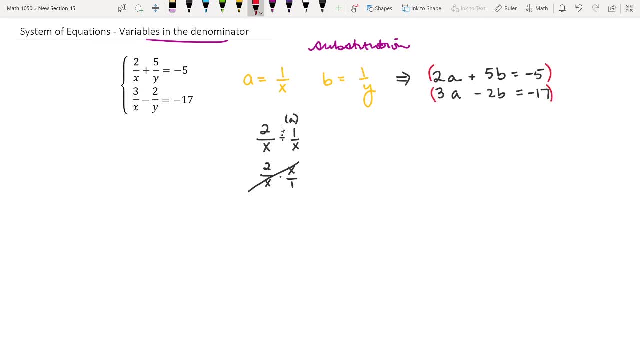 from previous videos that I've done. I like to focus on the x. It's something about being in the front. that just spots it in my head. These two have nothing in common, so I'm going to times them by each other And because they're both positive, I'm going to give 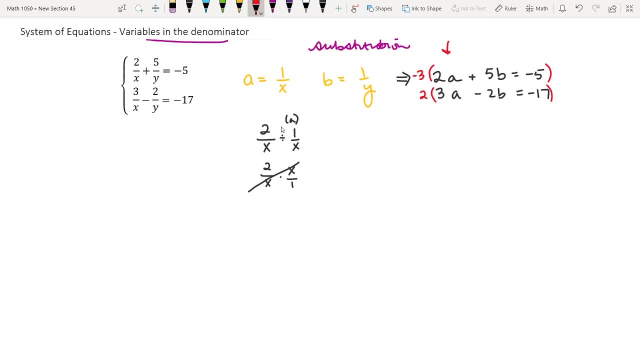 one, a negative. This time I'm going to choose that to be the top one. So I'm going to manipulate these equations so that I can have it work to my advantage. So I'm going to times that negative 3 through to all. 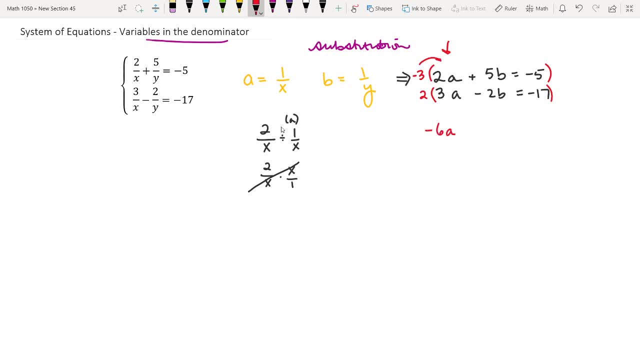 And I get the negative. 6a minus 15b equals 15.. And then I'm going to distribute my 2 through this bottom column and I have 6a minus 4b equals a negative 34.. Now, that's achieved what I wanted to do. 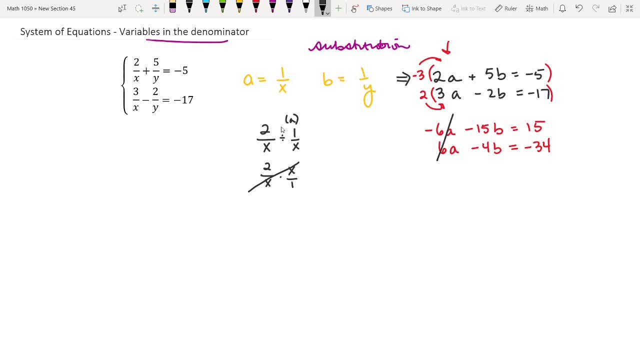 I wanted to get rid of 1 so that I can solve for the second variable, And that's the only way we can solve things. So doing so now gives me that negative 19b equals a negative 19. Which is perfect, right. Divide by a negative 19. 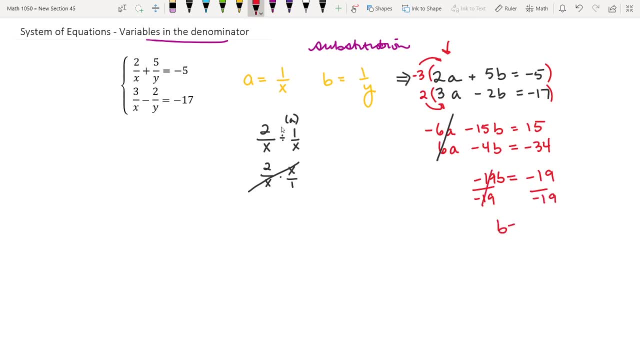 and I'm going to get that b equals 1.. Now for this. before we put things back in, because we do need to find the original x and y value- let's find a first before we put those fractions back in. So I'm going to put: 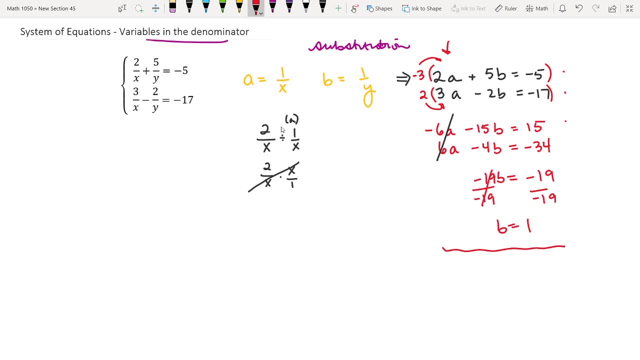 7p back in and, technically speaking, I have 4 choicesThe last two are a little larger than sometimes we want to deal with And the first two it doesn't make a difference, So let's go ahead and stick that b value back into the top one here. So I have 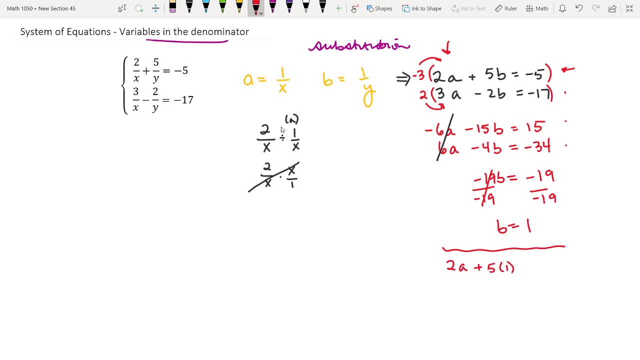 2a plus 5 times there's my b. put it back in And I can solve now for a. 2a plus 5 equals a negative 5.. I'll minus twice minus 5, I'll minus my 5 to both sides, and 2a equals a negative 10.. 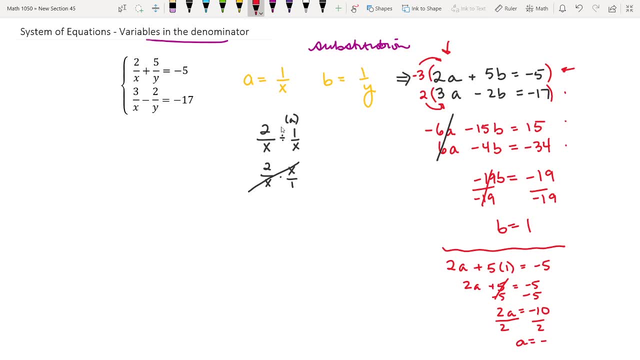 Divide by 2, and a is a negative 5.. So I've essentially found some values for my substituted variables. I now need to put those values back in, So we're going to come back over here and do so. So I had that a equals 1 over x, or if I put in this new value, 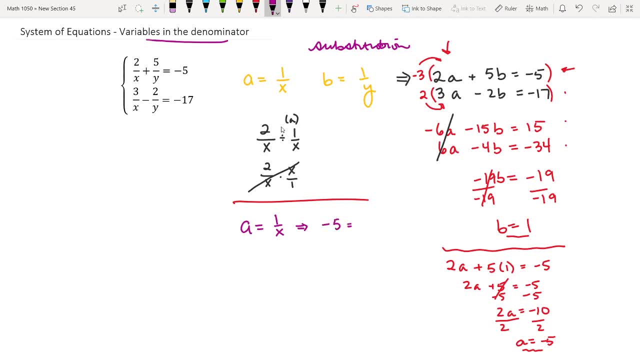 of a, I would say negative 5 equals 1 over x. Now, sometimes the easiest way to work with that, before you start thinking about common denominators, is go ahead and make them both a fraction and then think of it as a proportion, and I can cross multiply.